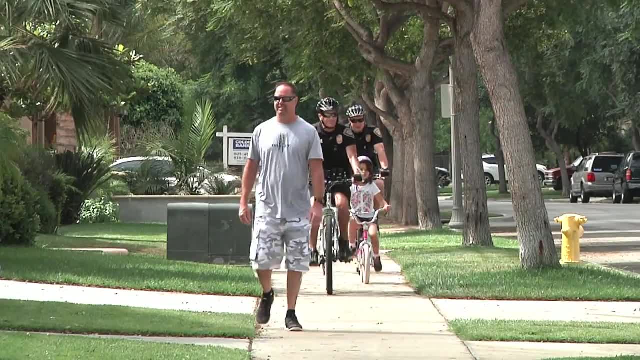 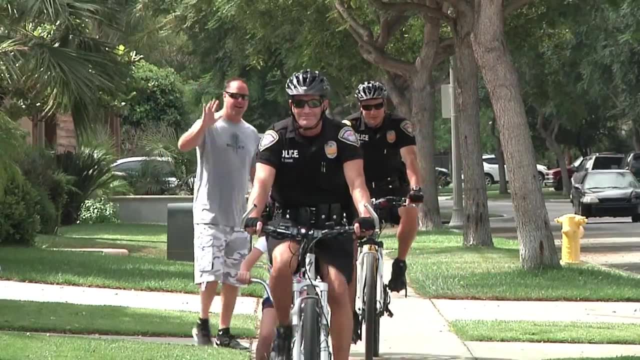 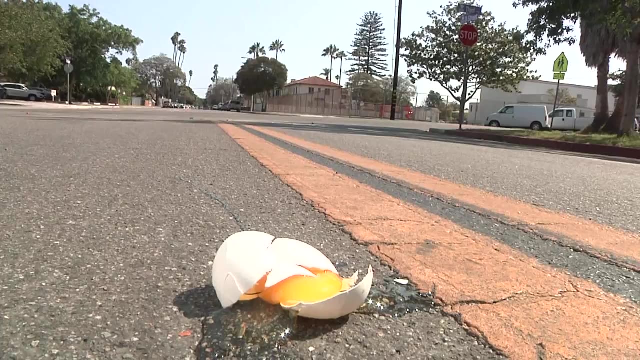 Alert pedestrians if you are passing them on the sidewalk by letting them know what side you are passing on. Make sure to wear your helmet. Your head is as fragile as an egg. It has a soft center with a thin shell. You need to protect your most precious asset from falls that could cause it to crack. 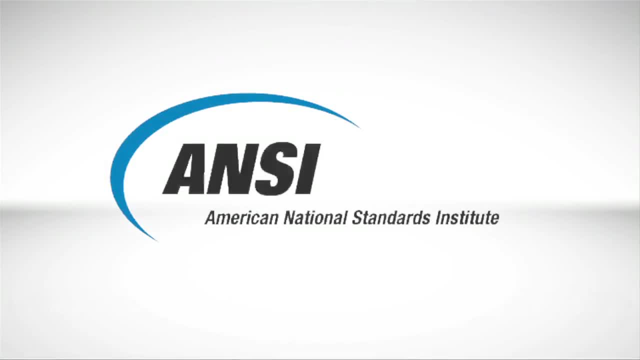 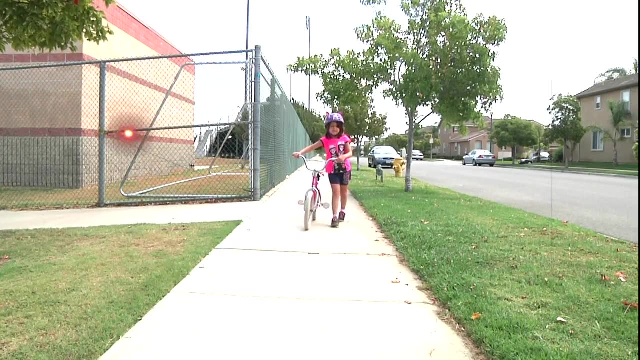 Remember to purchase a helmet. Use a helmet that is recommended by the American National Standards Institute, or ANSI. Replace your helmet if it has taken a blow of significant impact. When riding in the roadway, wear clothing that increases visibility in traffic. Use lighter, brighter colored but close-fitting clothing so as to be seen much more easily. 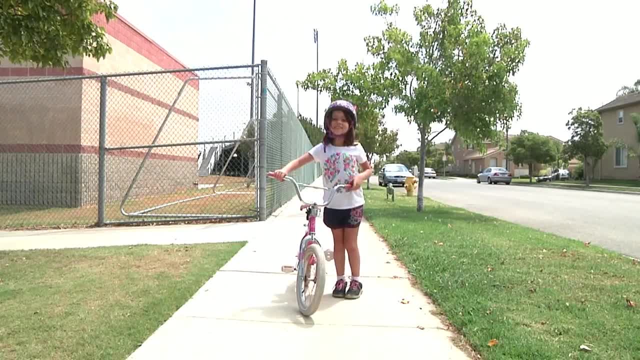 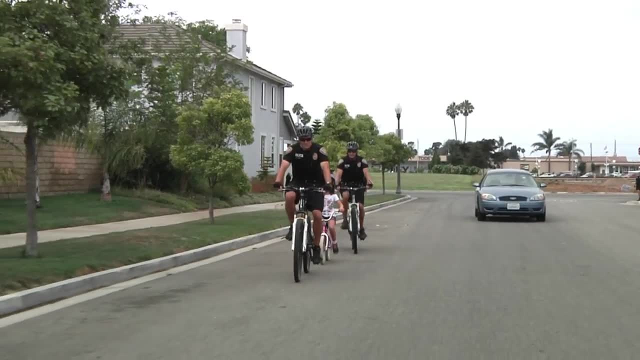 by traffic. Make sure that it is clothing that will not become entangled in the gears or crank of a bicycle. Go with the flow of traffic. It is against the law to salmon ride, which is riding against traffic. Warn traffic when stopping or turning. 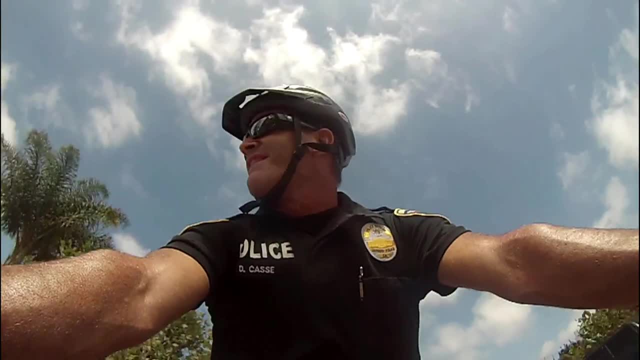 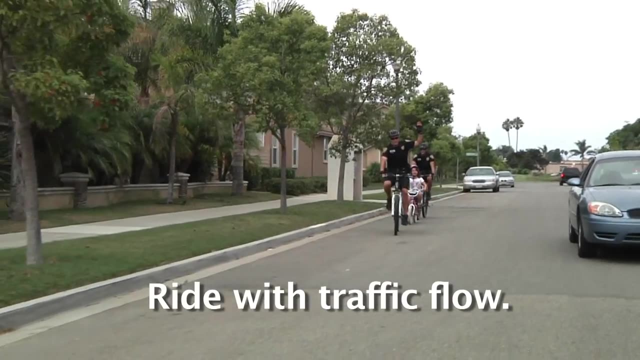 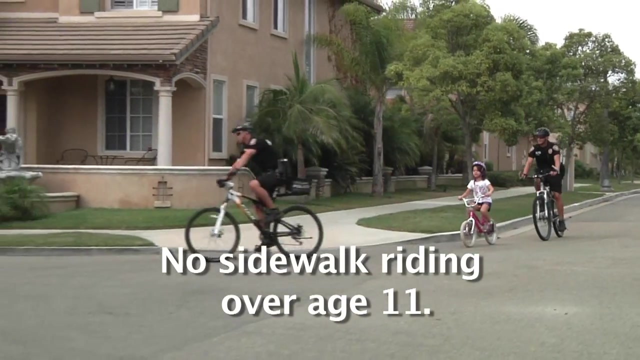 A bicycle is considered a motor vehicle when it is on the roadway and must follow the rules of the road. Some rules that apply to bicyclists are: riding with the flow of traffic, no salmon riding, needing headlights at night, no riding on the sidewalk if you are over the age of 11,. 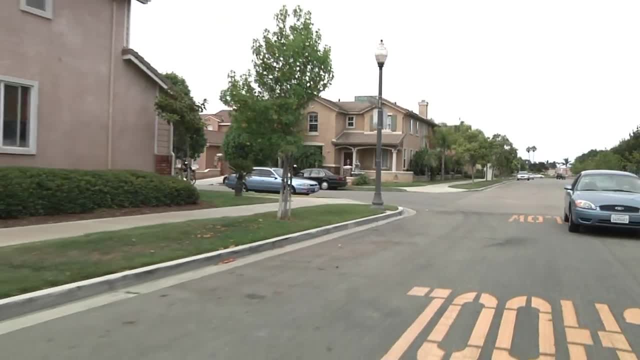 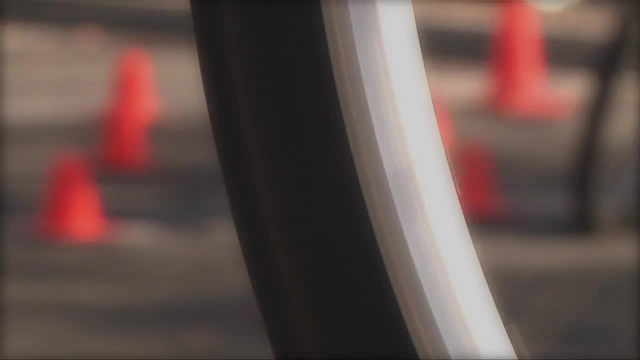 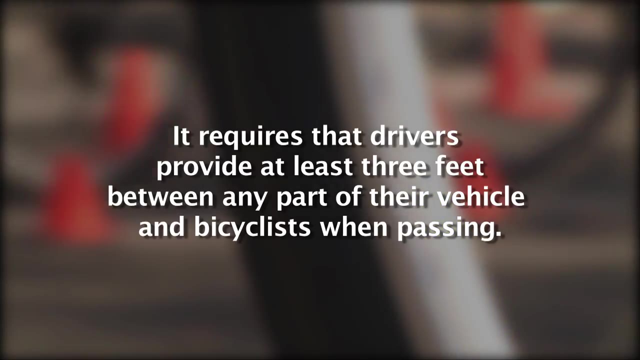 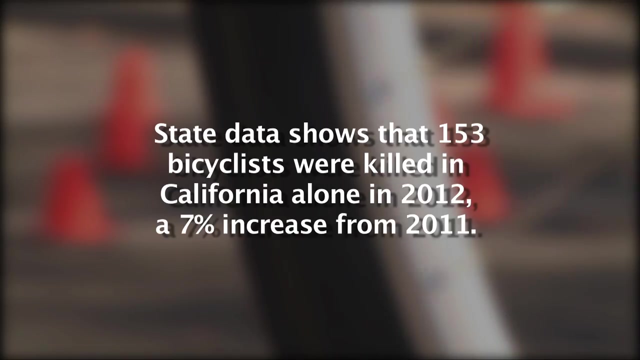 no hitching rides or riding double. except on bicycles built for two persons. The rider is allowed to turn in the direction of the roadway and must ride with all the gears and gear available. By using the velcro strap, you can make a partial and close-fitting understanding of 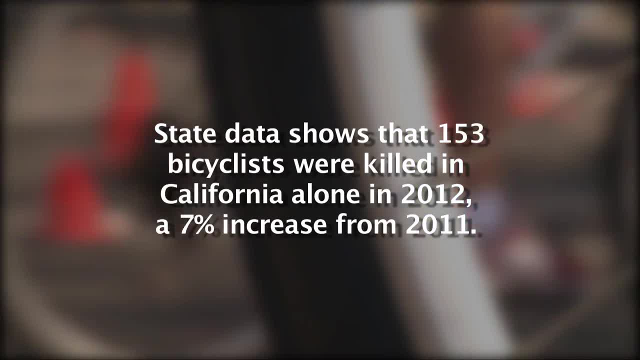 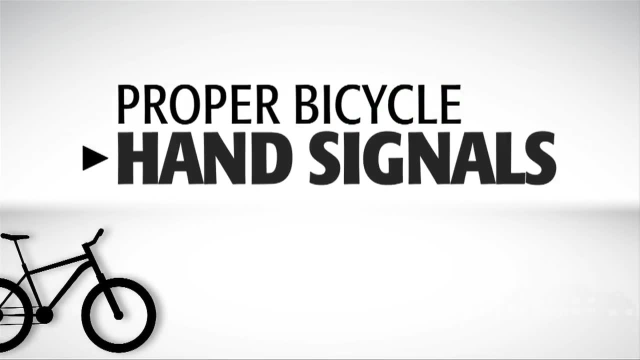 the road and the road surface. Finally, if you have a moped with speed, sometimes a bicycle can be used as a guide for the road to reach a road where you can safely ride on the road. The bicycle is παси. the bicycle isread. the bicycle is read. the motorcycle is read. the. 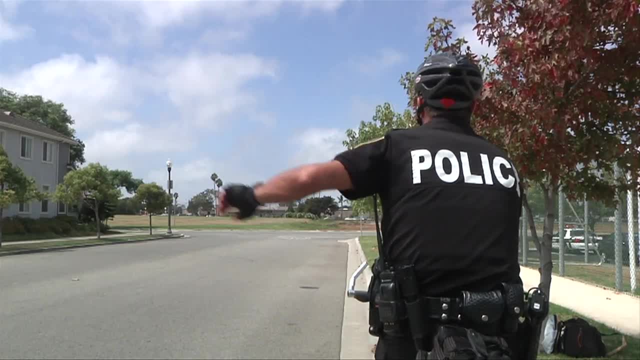 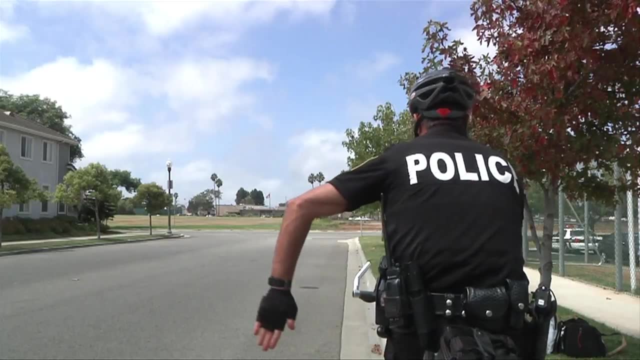